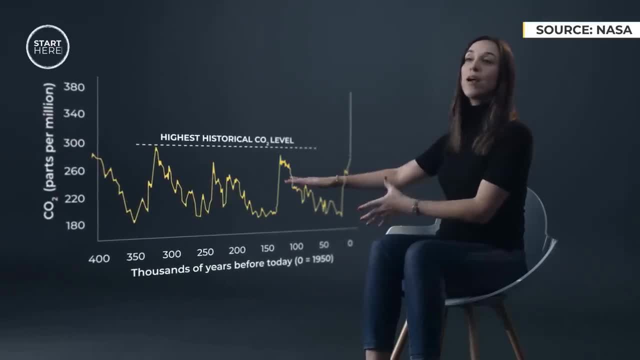 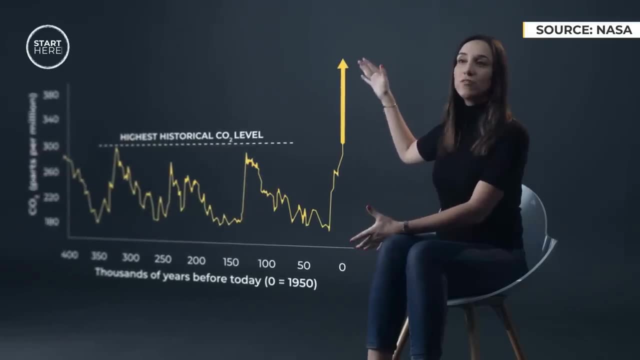 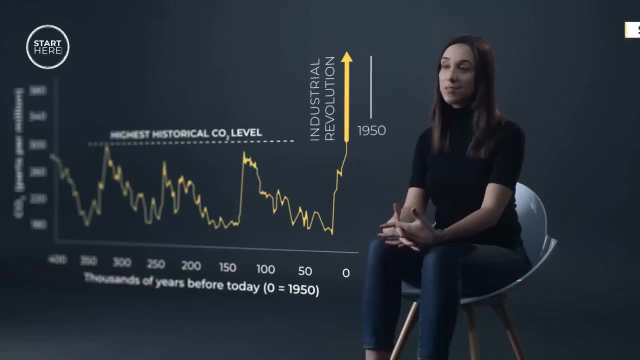 Look at this graph. These are the levels of carbon dioxide in our atmosphere over hundreds of thousands of years. But this spike in carbon dioxide at the very end, that took off during the industrial revolution. We started breaking CO2 records in 1950 and we haven't stopped since. 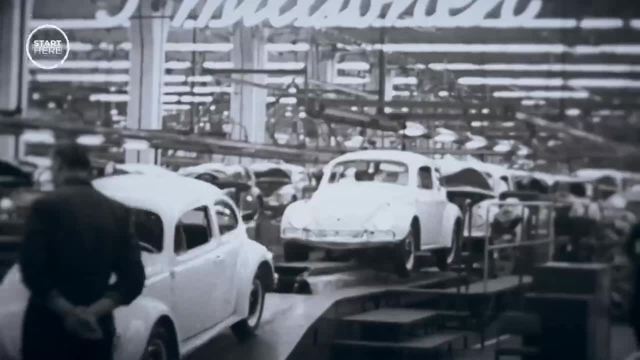 Why? Well, scientists say there's a 95% chance that human activity is the cause. 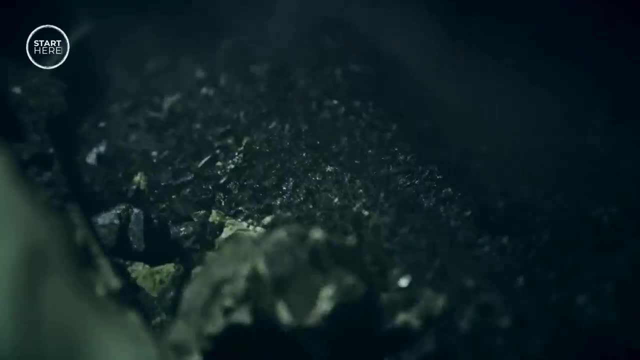 We've been burning more and more fossil fuels like oil and coal, which release CO2, to power our homes, factories, airplanes and cars. 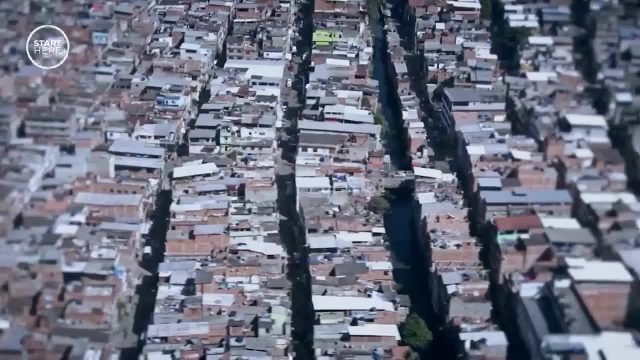 There's also a lot more of us. The global population has tripled in the past 70 years. 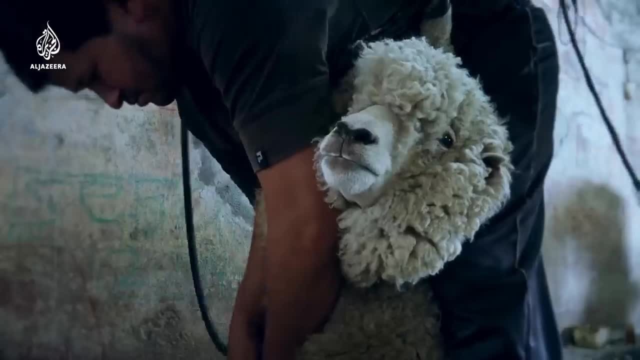 And we're consuming more products from animals that release another pollutant called methane. 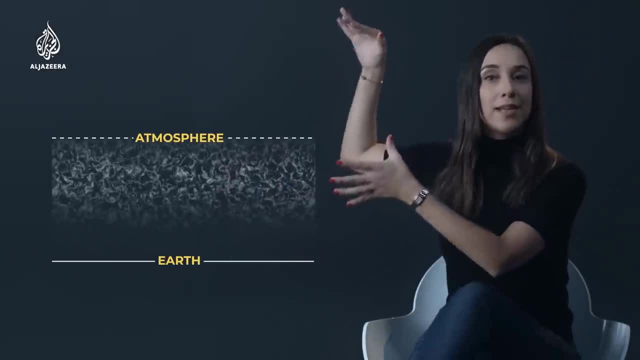 So, all those gases are released into the air. And when sunlight gets into the Earth's atmosphere, some of the heat gets trapped and the planet gets warmer. That's why they call it the greenhouse effect. 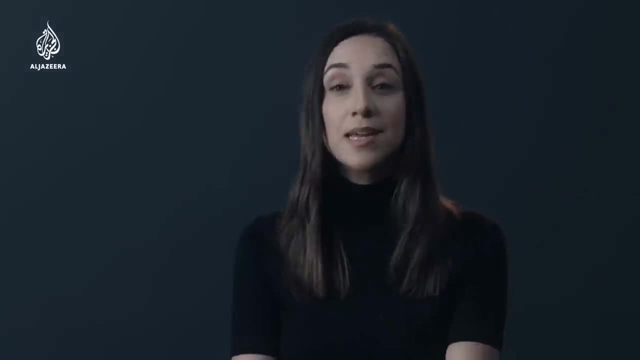 But the concern is not that the earth is getting warmer. It's that it's happening far too quickly. 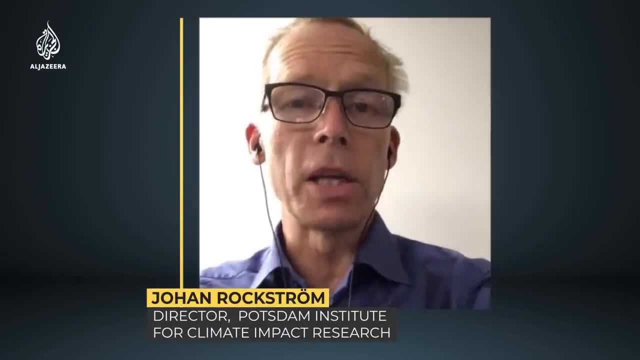 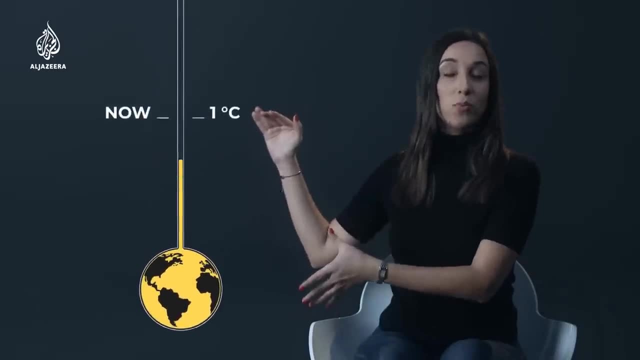 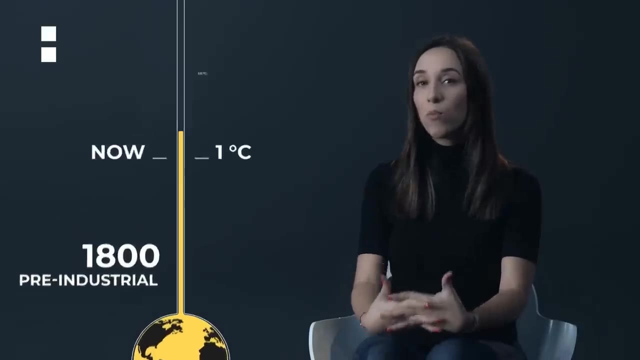 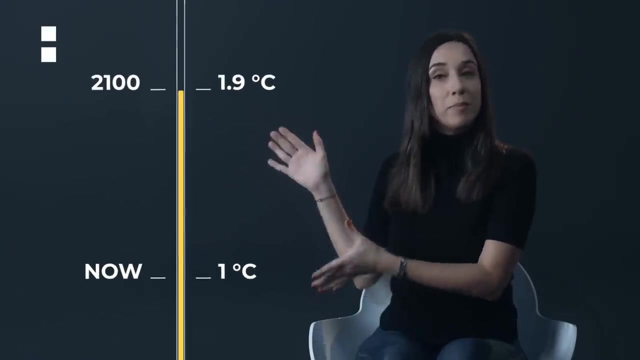 But it's actually the warmest temperature on Earth since the last Ice Age, since 10,000 years ago. The UN says that right now, our world is about one degree hotter than pre-industrial times. That's around the year 1800. Which is okay. In fact, the UN says if we warm by 1.5 degrees before the end of the century, we should be fine. The UN even says 2 degrees would probably be alright. 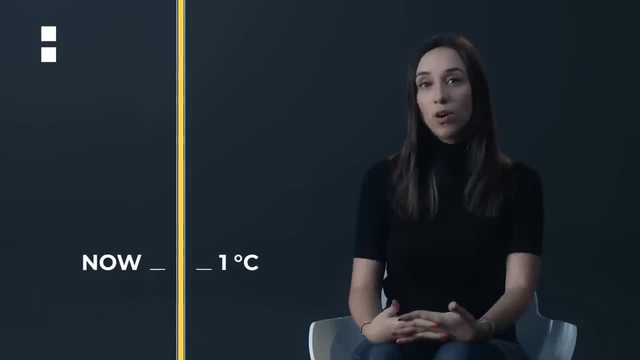 But again, the problem is speed. Because right now, we're on track to hit 1.5 degrees in only 10 years. And if we don't slow that warming down, it could mean catastrophe within my lifetime and maybe yours too. 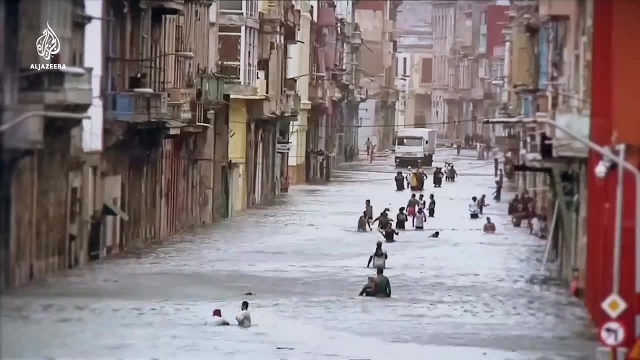 And we're already getting a taste. Climate change is here. Climate change is happening. 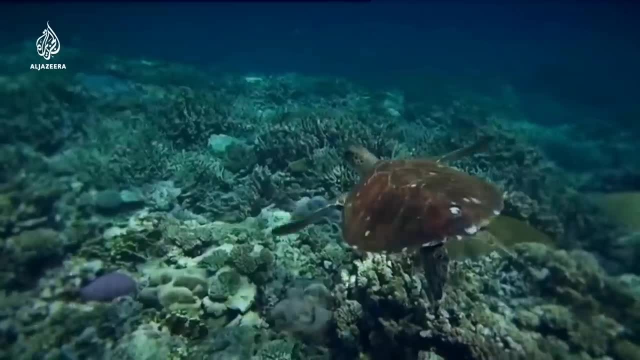 We are well into the sixth mass extinction event. Europe is currently colder than the Arctic. 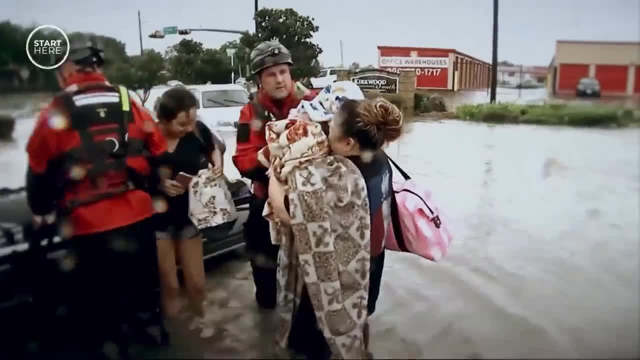 More than a thousand people being rescued just in the early morning hours of Sunday. Millions of people are likely to die. Millions of people are likely to suffer worsening food and water shortages. 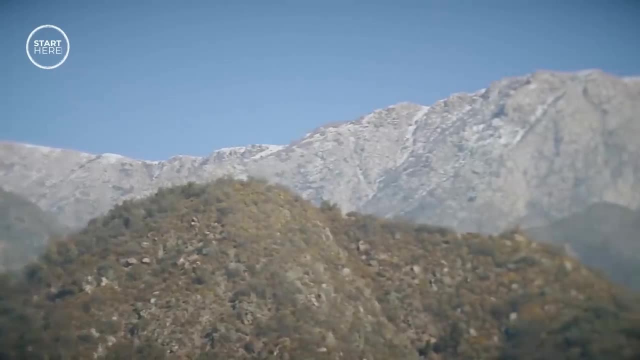 Drought, which is now in its tenth year, is a phenomena that's here to stay. We've never seen a year's worth of rain in less than seven days. Sea levels are rising about three millimeters a year because sea water expands as temperatures get warmer. 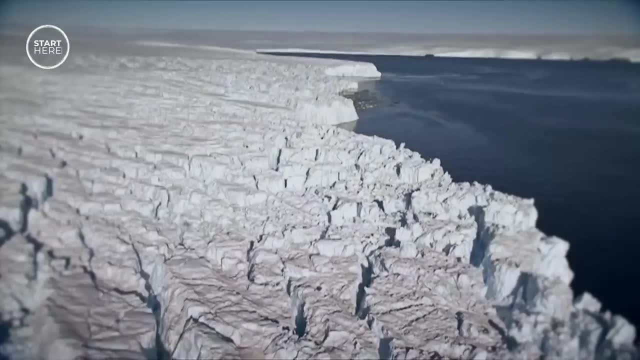 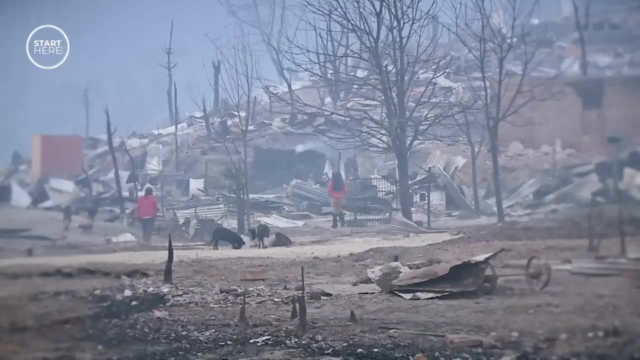 Melting ice sheets and glaciers also add trillions of tons of fresh water into our oceans. People around the world are already losing their homes. 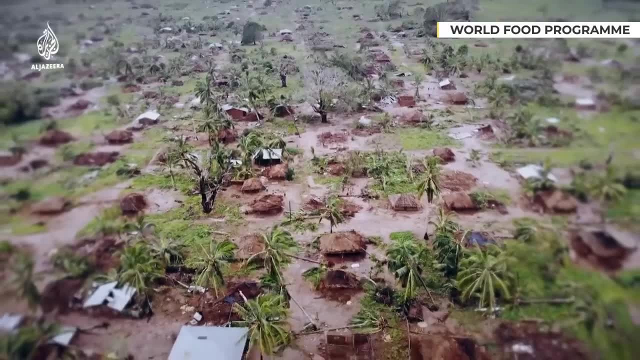 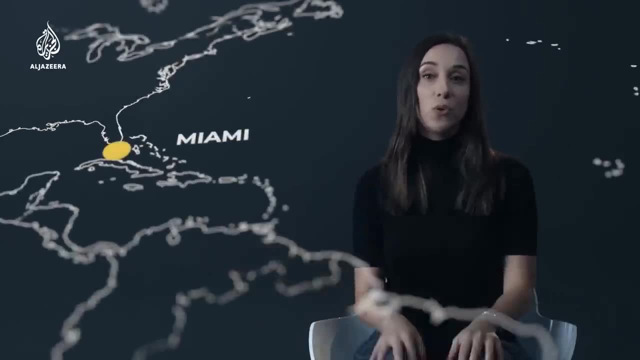 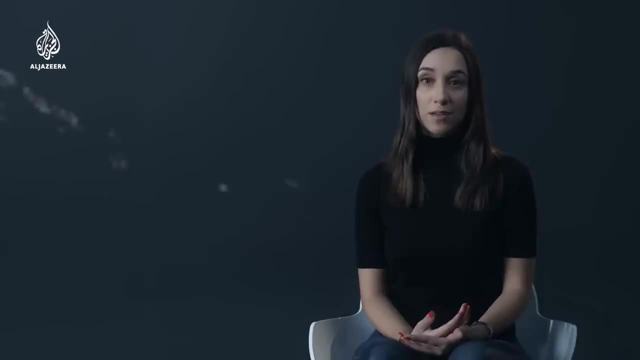 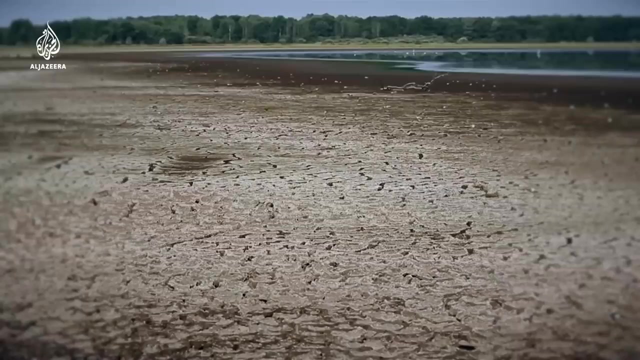 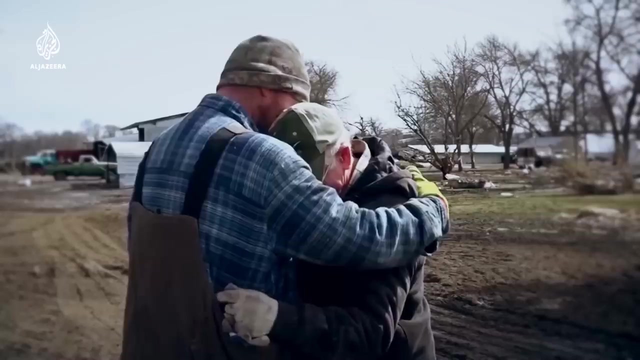 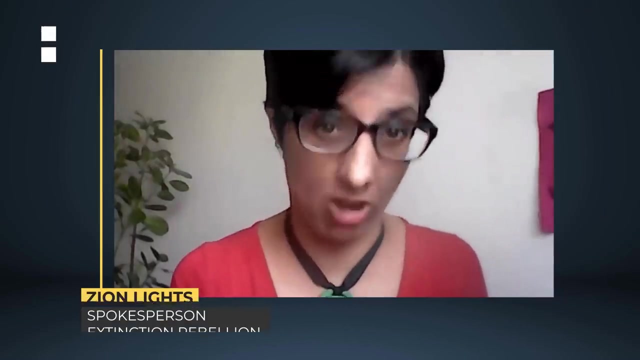 And if things carry on, millions more of us will have to pack up too. Entire coastal cities could be underwater within 80 years, like Miami in the U.S. or Osaka in Japan. Entire island nations in the Pacific could completely disappear. Natural disasters becoming more and more intense, more frequent, with more devastating consequences. The dramatic impacts of drought in different parts of the world. All this is creating a situation that is a real threat to humankind, and we are not doing enough. If 99% of doctors said to you, take this medicine or you will get really sick and probably die, you would take it. Who wouldn't take it? The problem is, at the moment, we don't have any medicine. 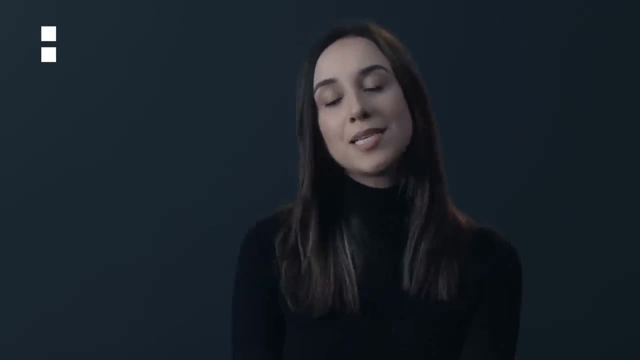 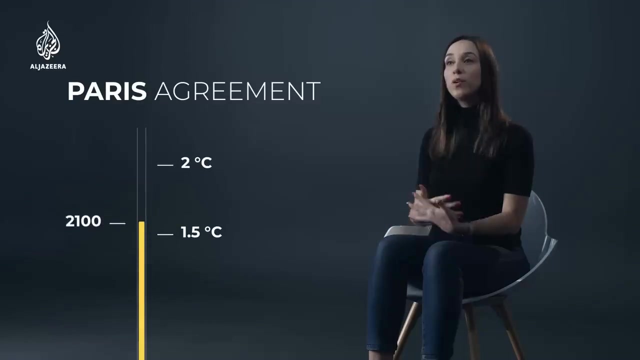 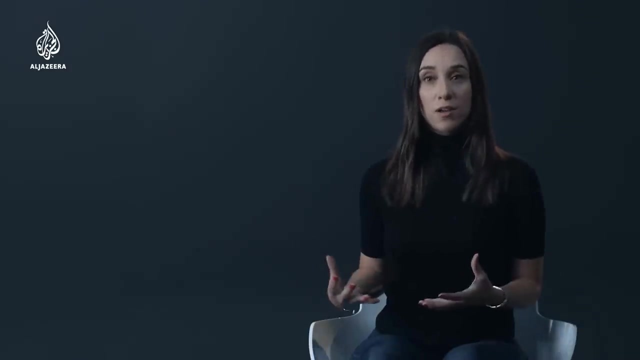 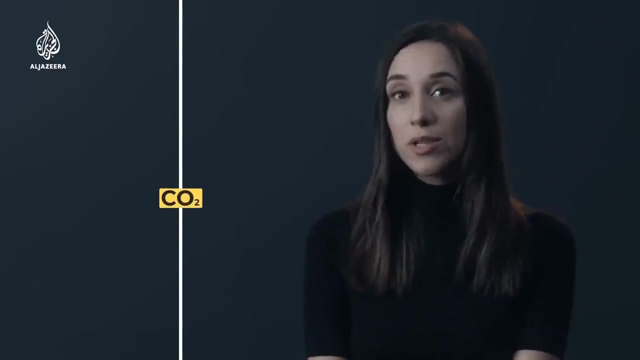 Now there is a plan to slow all this down. Back in 2016, world leaders signed the so-called Paris Agreement, and the big pledge is to cap temperatures rising by 1.5 degrees. Or a maximum of 2 before the year 2100. So countries set their own targets on how much CO2 they emit. But here's the thing, three years after the agreement, global CO2 levels are still going up. CO2 emissions have been going up the last year by 2%, so that's actually above the average of the last 10 years. 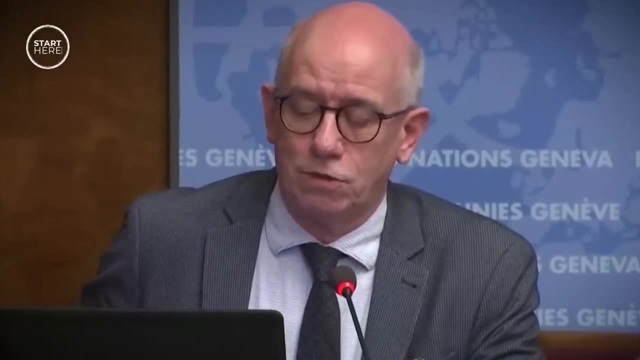 So it's started to increase again, and it doesn't look too good. In some ways, we're going backwards. 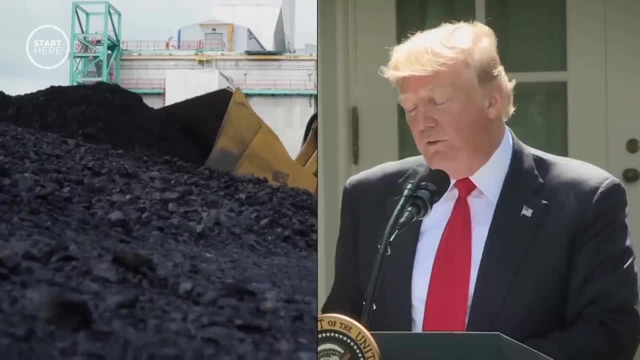 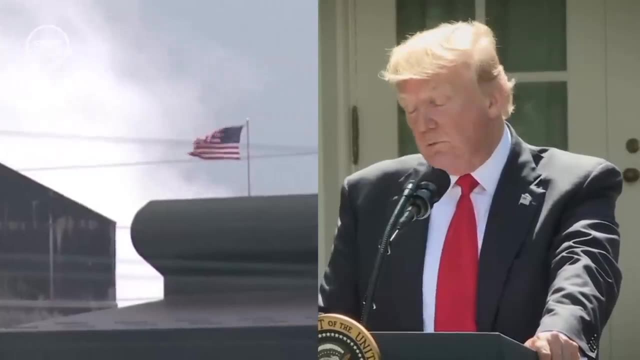 The United States will cease all implementation of the non-binding Paris accord, and the draconian financial and economic burdens the agreement imposes on our country. 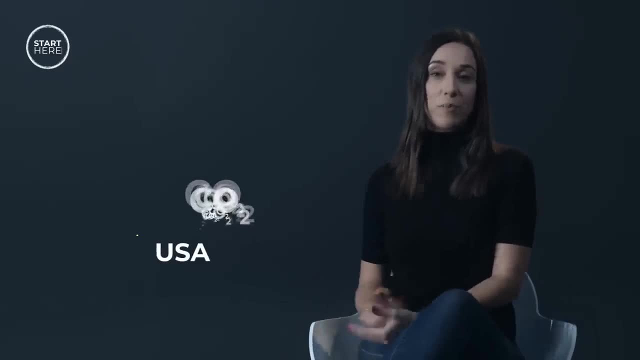 The US, one of the world's biggest polluters, has pulled out of the Paris deal. 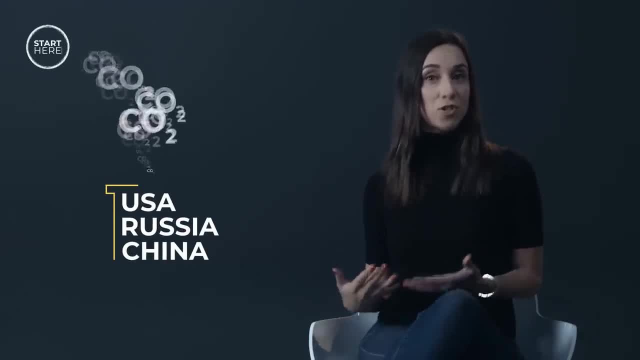 Russia and China are accused of not giving themselves ambitious targets in the first place. 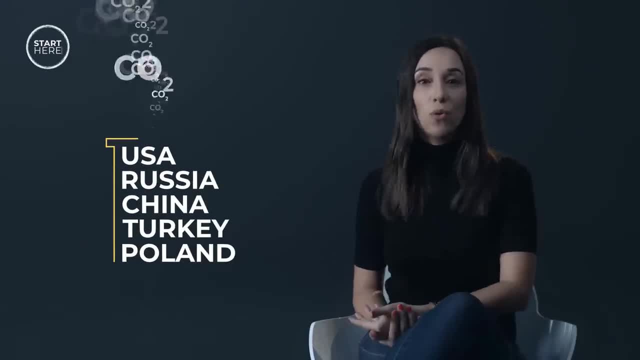 Turkey and Poland want to build more power plants that use coal. And then there's the skeptics. It's a political decision.